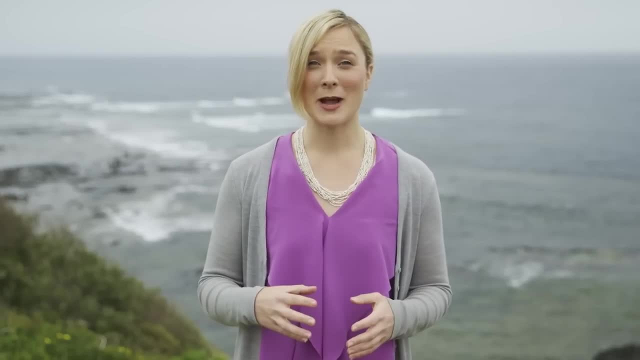 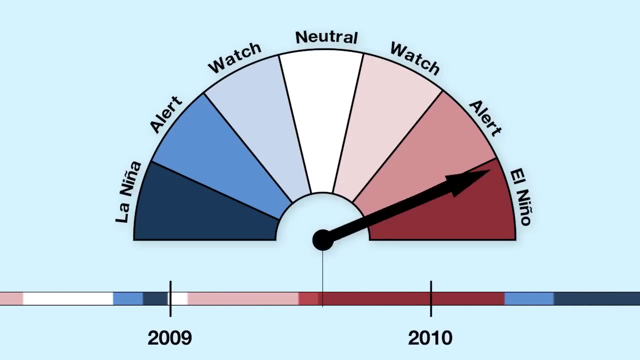 Neutral and El Niño. A typical ENSO phase starts in the first half of the year and lasts until the following autumn. Sometimes we can get the same phase for two or more years in a row. On average, it takes about four years to. 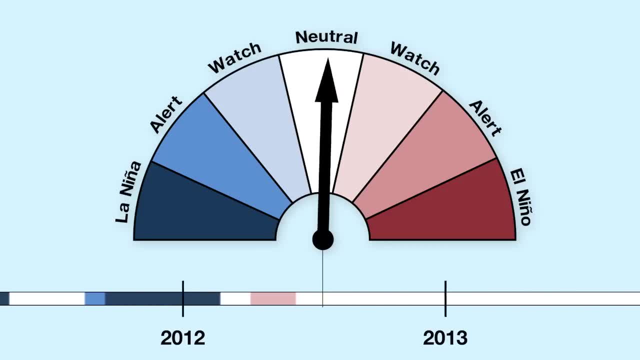 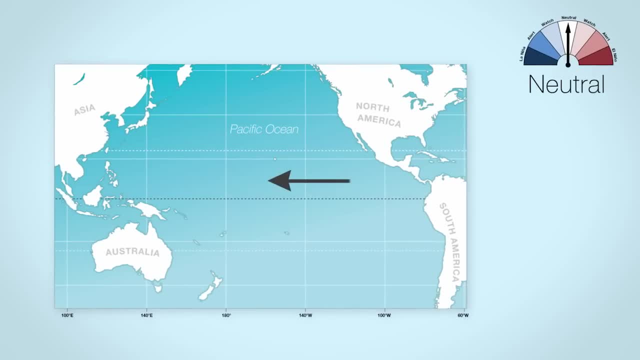 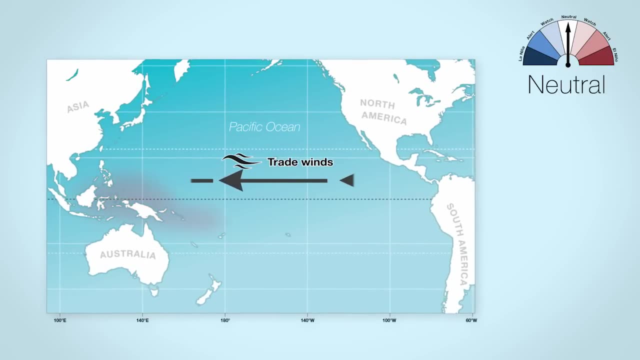 swing from El Niño to La Niña and back again. So what are these ENSO phases and how do they impact Australia's climate? Well, during the neutral phase, steady trade winds blow across the tropical Pacific from the east to west. These winds pile up warm water in the western Pacific, In contrast, water temperatures 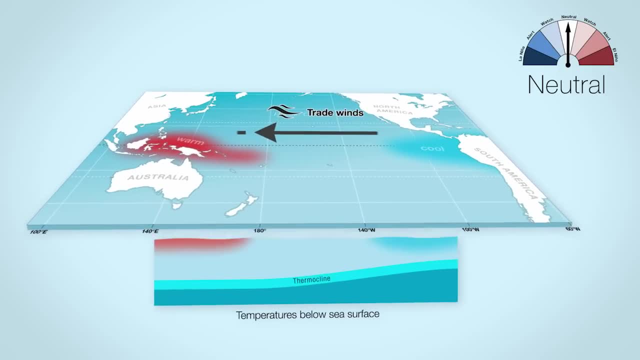 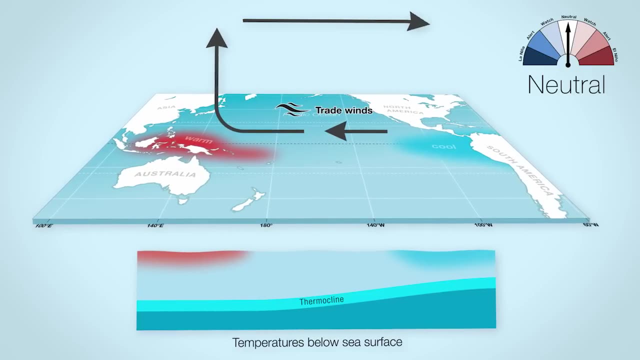 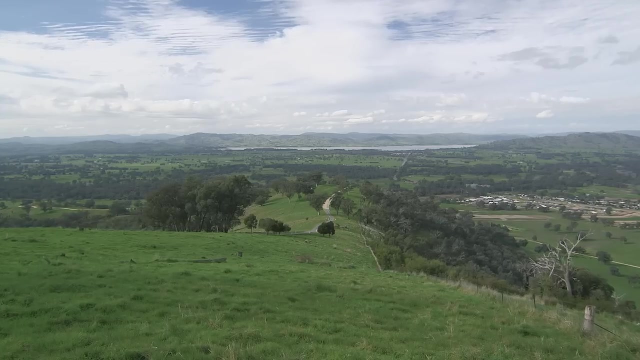 rise in the north as the trade winds cause cool water to be drawn up from the deep. The temperature difference across the tropical Pacific Ocean causes air to rise to Australia's north and descend near South America. This creates a huge connected cycle called the Walker Circulation. We consider neutral to be. 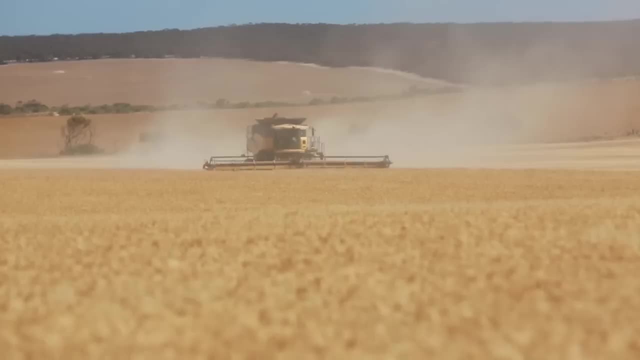 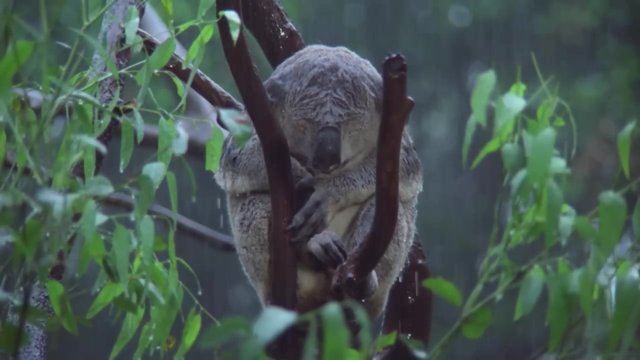 the normal phase because we're in this state more than half of the time. While a neutral phase may bring more normal weather to Australia, droughts and floods are certainly still possible. When we move into El Niño. it's a bit like the neutral phase has gone into overdrive. 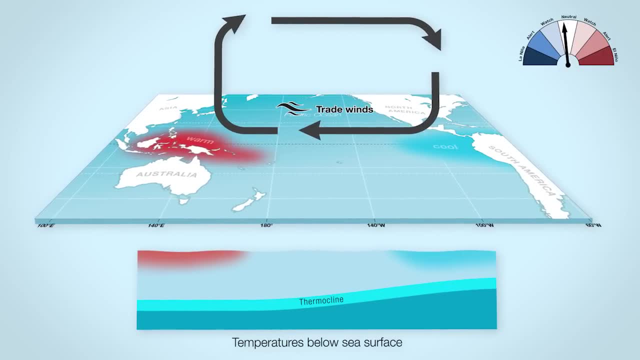 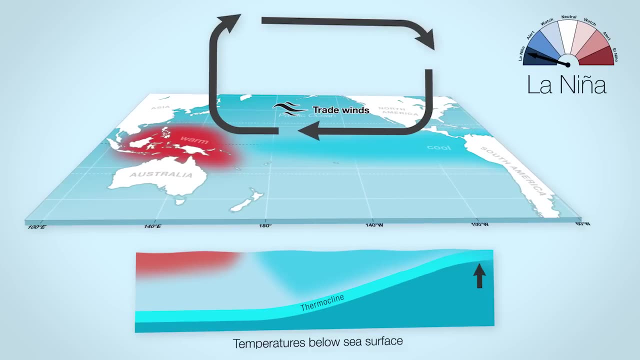 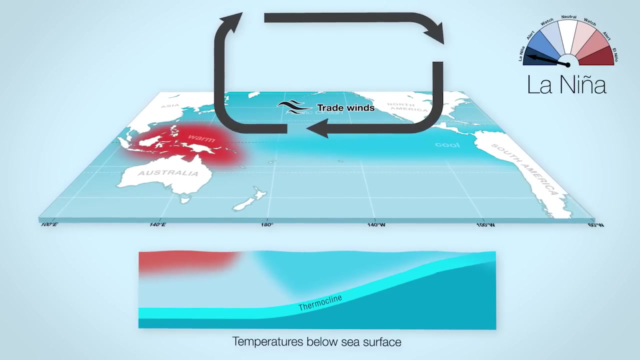 The trade winds blow harder, expanding the warm pool on the Australian side of the tropical Pacific and cooling the oceans towards South America. This increases the east to west temperature difference and makes the Walker Circulation even stronger and the trade winds blow even harder again. This is called a feedback. 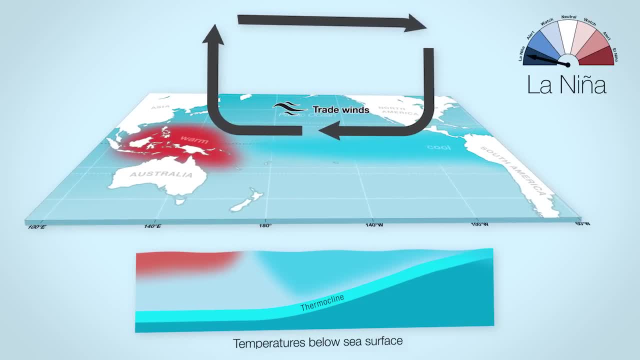 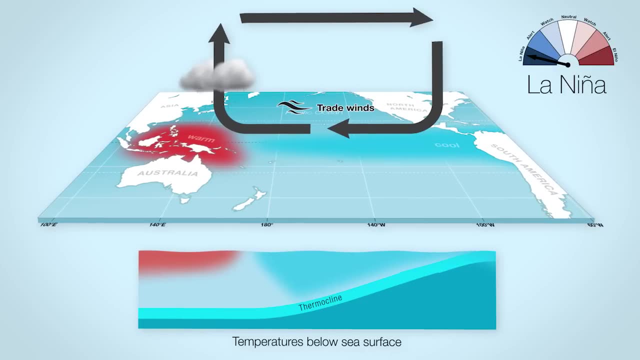 loop and once it starts we're locked into El Niño until at least the following autumn. With the higher ocean temperatures, we get greater evaporation, more cloud and more rain in the western Pacific. For Australia, this means a higher risk of widespread flooding. 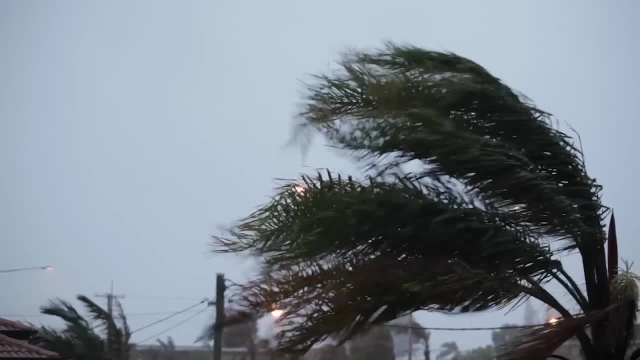 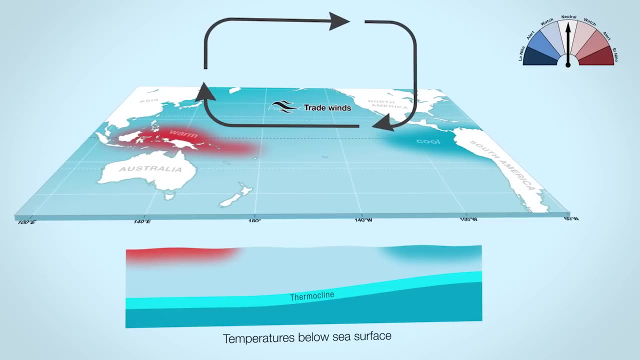 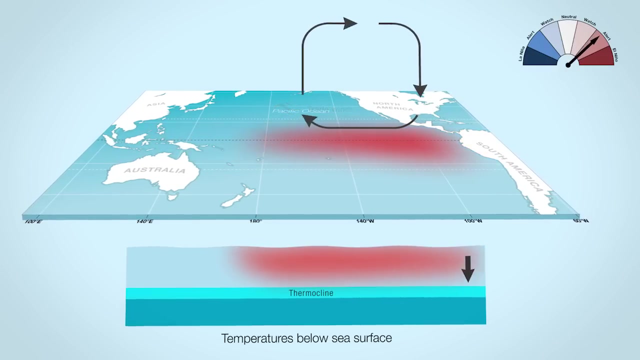 lower daytime temperatures and more tropical cyclones. On the other end of the scale, we have El Niño, which is almost the direct opposite of La Niña. During El Niño, the trade winds actually weaken or reverse, allowing warmer waters to drift back Towards the east. the change in the ocean temperature patterns mean the Walker Circulation breaks down.